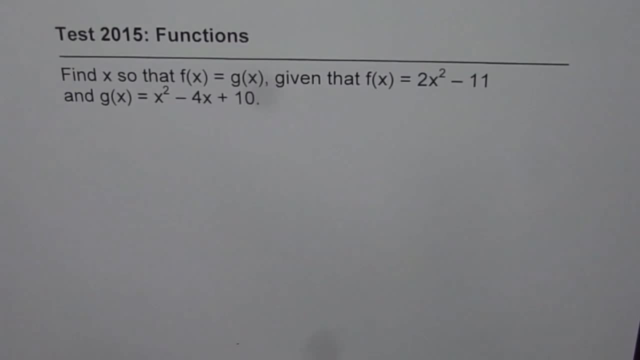 Here is question number 3 from test 2015 on functions for grade 11.. Find x so that f of x equals to g of x. given that f of x equals to 2x square minus 11 and g of x equals to x square. 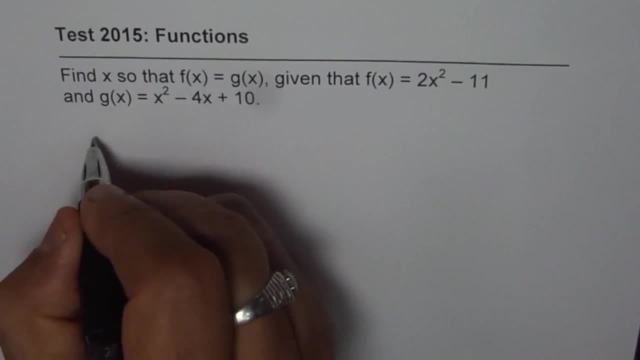 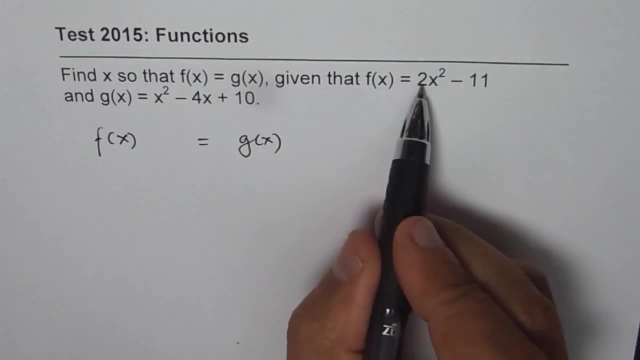 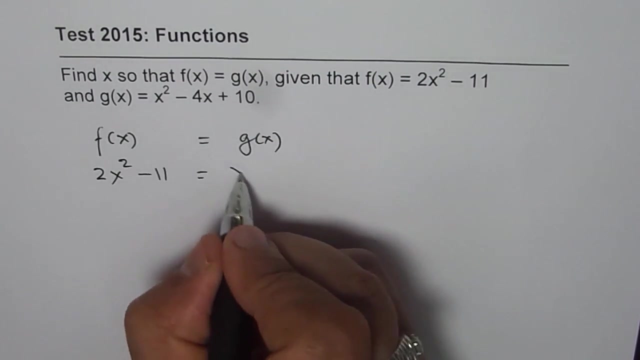 minus 4x plus 10.. Now we need to find the value of x, for which f of x is equal to g of x. f of x is 2x square minus 11.. So we can write: 2x square minus 11 equals to g of x is x square minus 4x. 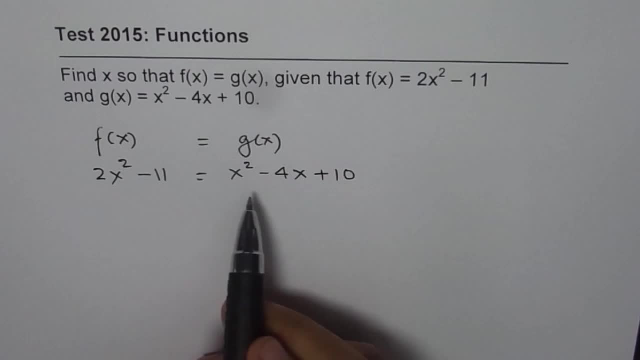 plus 10.. Now to find the solution, let's bring all the terms to the left, So we have 2x square minus 11 minus x square plus 4x minus 10 equals to 0.. 2x square minus 11. 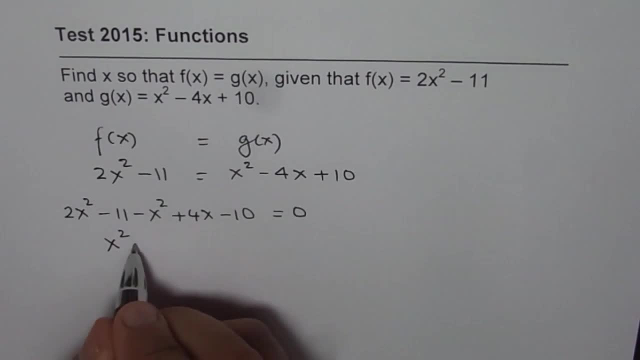 minus x square is x square. plus 4x minus 11 and minus 10 is minus 21, equals to 0.. Now we can factor this quadratic equation. We are looking for two numbers whose product is minus 21 and sum is plus 4.. So the numbers are 7 and 3,. 7 with positive sign, 3 with negative sign. 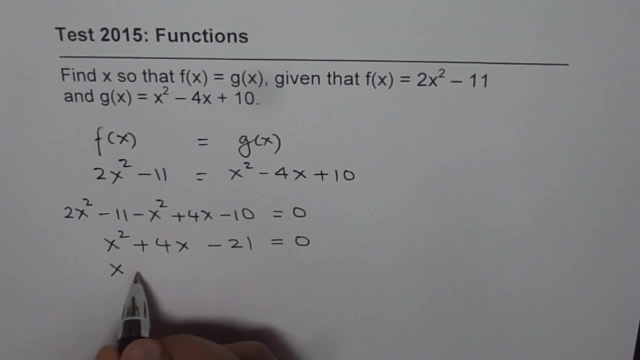 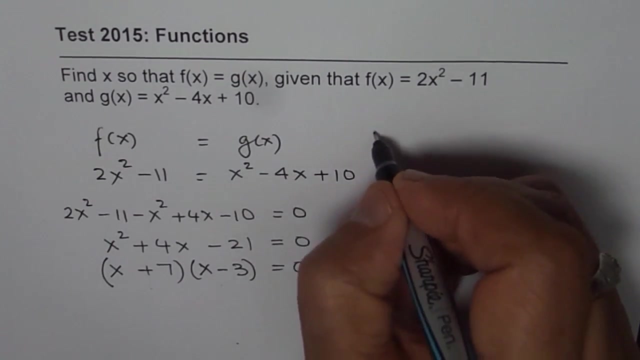 so that they add up to plus 4.. So we can factor this as: x plus 7 times x minus 3 equals to 0.. Now that gives us two solutions, right, So to get the solutions, we need to equate each factor to 0, right, So equating x plus 7 to 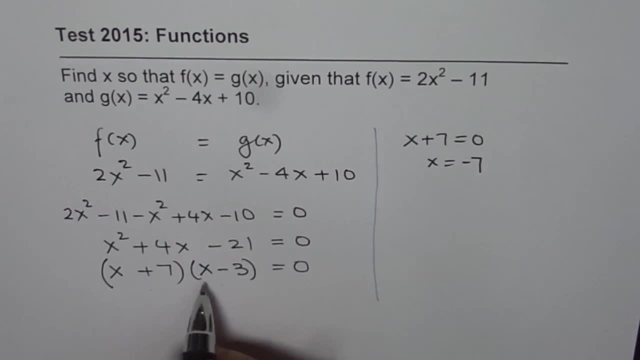 0 gives us x equals to minus 7, and equating x minus 3 equals to 0 gives us x equals to 3, correct? So there are two points. Answer is: add x equals to minus 7 and x equals to 3.. But remember one thing: 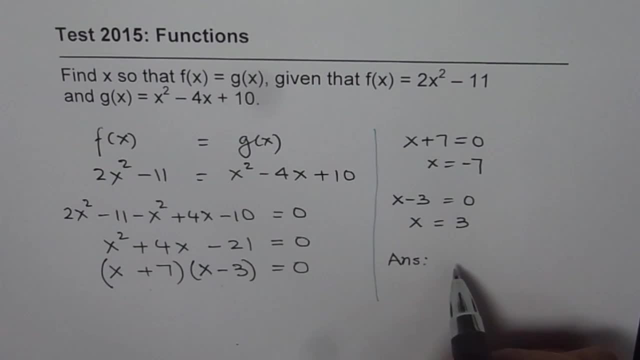 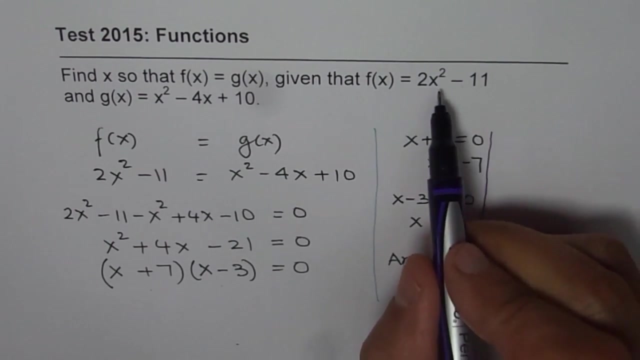 When we are giving coordinates of a point, we should actually give y values also, right? So let us find out the y values of the function at these points, right? So at x equals to minus 7, what is y value equals to? So we'll substitute minus 7 here, right? 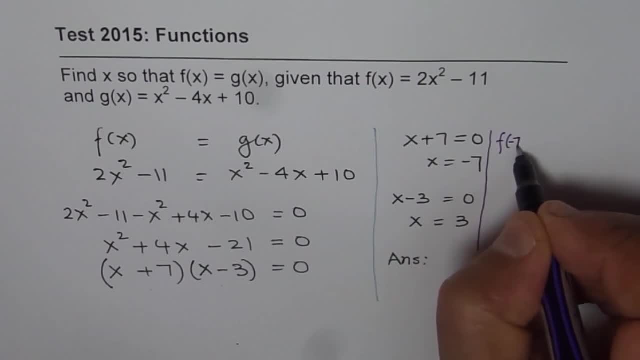 So let me see: f of minus 7 equals to 2 times minus 7, square minus 11,. right, That means 2 times 49 minus 11,. 2 times 50 is 100, so it is 2 less, so it is 98 minus 11, and that gives us 87.. 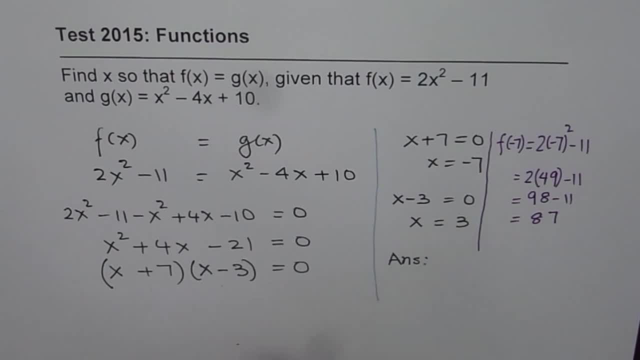 So the first point for us is: let me write down answer here now. So the first point for us is: minus 7, and 87 is a y value. Now the second point is: when x is 3, right. 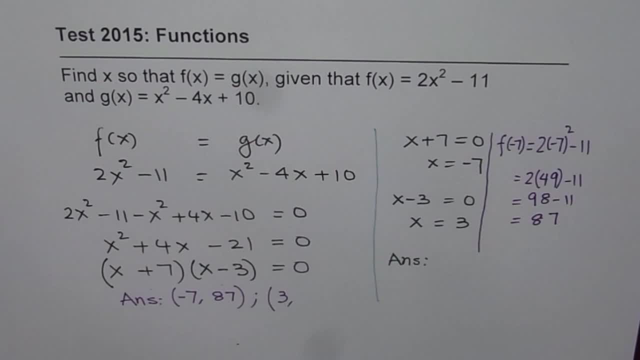 So x is 3, so let's substitute 3 now in the given equation and find the value of y. You could use any of these equations, it doesn't really matter. these are point of intersection, right? So they have to be same. 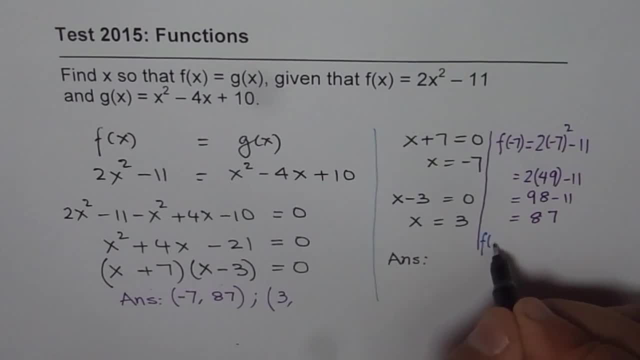 Let me use the first itself. So we have f of 3 equals to 2 times 3 square minus 11, which is 2 times 3 square 9, 9 times 2, 18, 18 minus 11 will give us 7.. 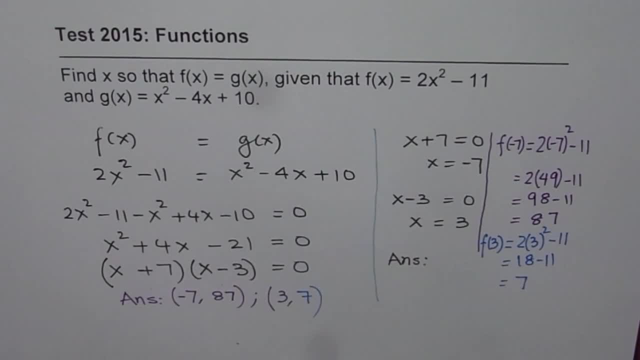 So the y point is 7 for you, right? So we have these two points where the function will intersect, right? But the question was only find x, so that this, so the x values which we got, were correct. 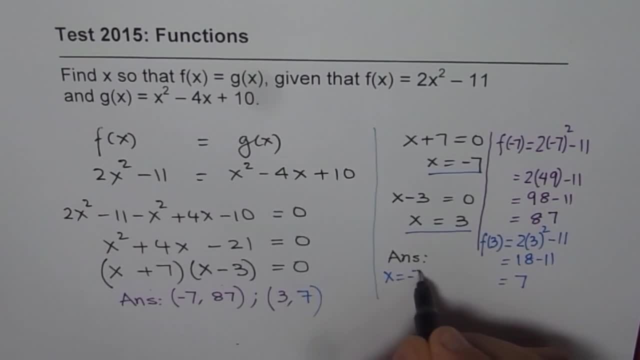 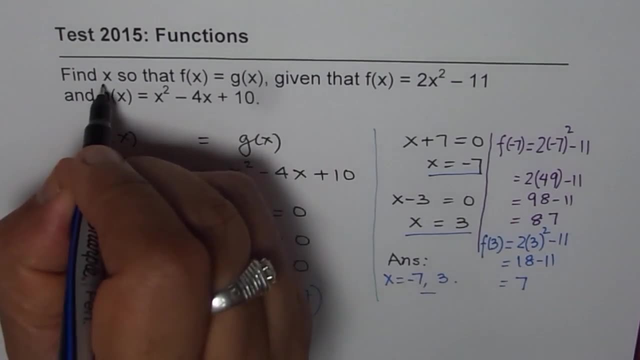 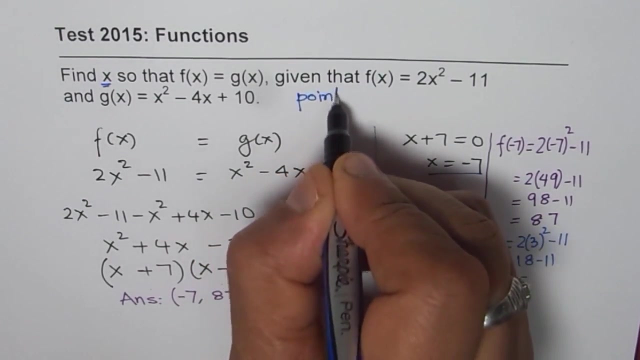 and we can write down The x values. are x equals to minus 7 or 3, right? So I just did this, in case we change this question from find x to find coordinate points. right, Find coordinate points, or find points so that f of x equals to g of s. 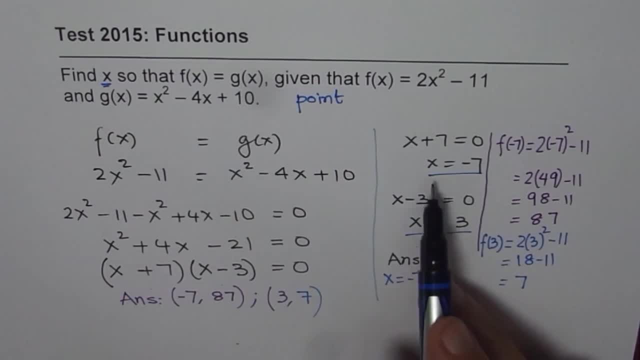 In that case you have to do this part, Otherwise that is the solution and you know you don't have to do that part, right? I think that helps. Thank you and all the best.